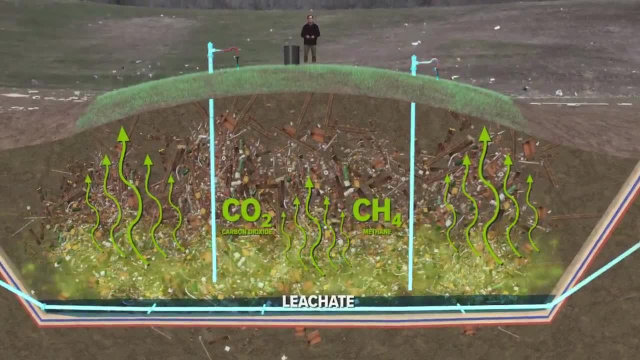 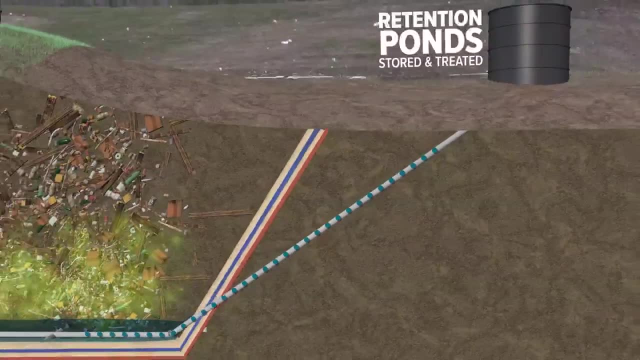 on top of the leachate. Landfills have a system to collect both the leachate and the gas so they don't contaminate the environment. Pumps send the leachate to retention ponds where it's treated and stored. There are also vertical gas wells running down through the landfill. They 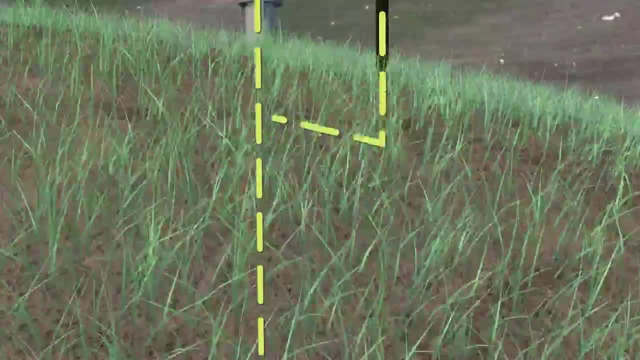 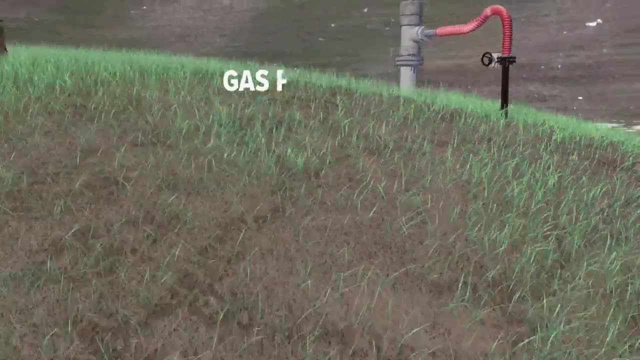 get pumped and stored in a tank to collect the leachate. When the gas comes out of the use vacuums to collect the gas. Different pumps inside those wells send the gas up and out to a gas plant where it can be processed and sold as usable natural gas. Now, if these 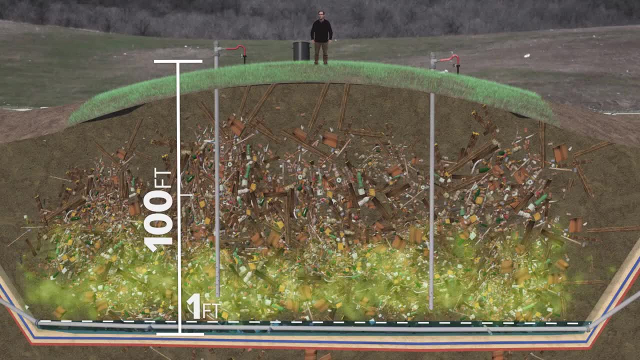 pumps are working properly, there should be only one foot of leachate under that 100-foot mound of garbage. The vacuums that suck the gas into the wells sit right above that normal leachate level. But if the pumps are not working like they were in a Jefferson Parish landfill, 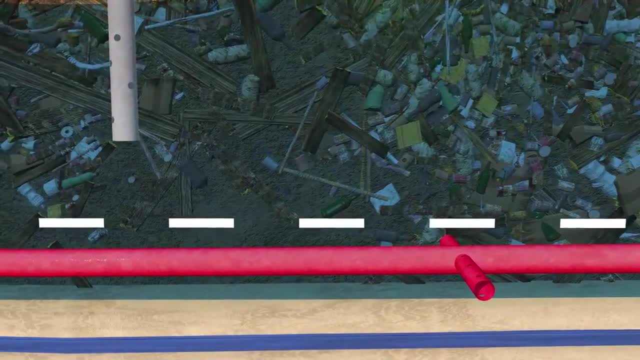 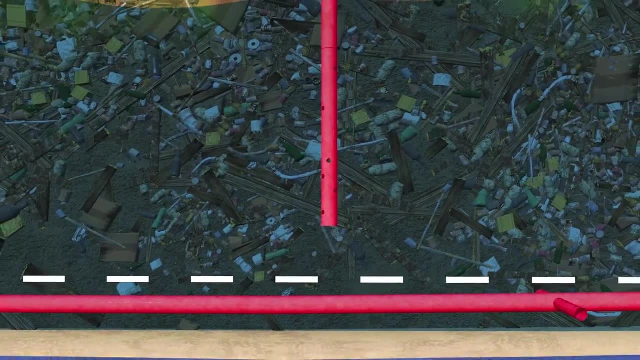 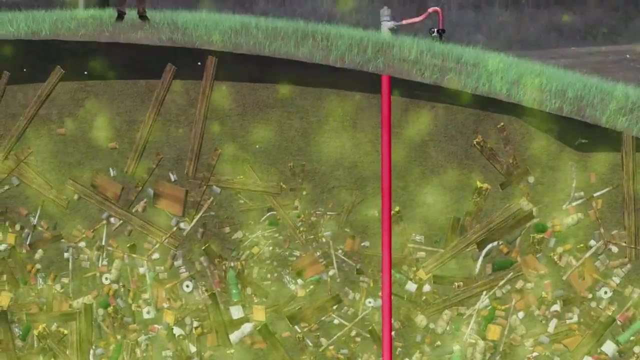 for years, the mound of garbage becomes flooded with leachate. That flood of leachate can block the vacuums from sucking the gas into the wells, and now that layer of toxic, smelly methane and hydrogen sulfide isn't being collected anymore. Instead, it rises up through the landfill and escapes into the air. 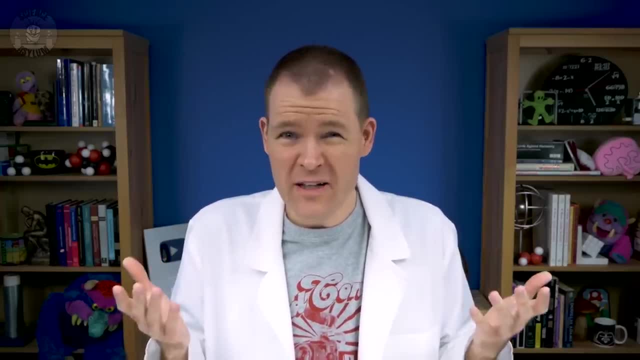 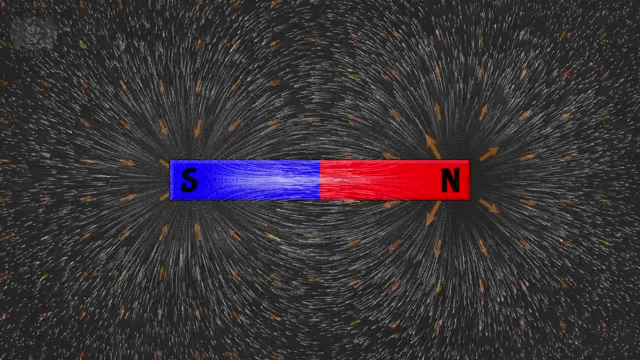 Hey Crazies, Sometimes math is unavoidable. Without it, you miss out on important insights. So what if, instead of avoiding math, we try to visualize it? I want to give you a glimpse inside my head for a few minutes.